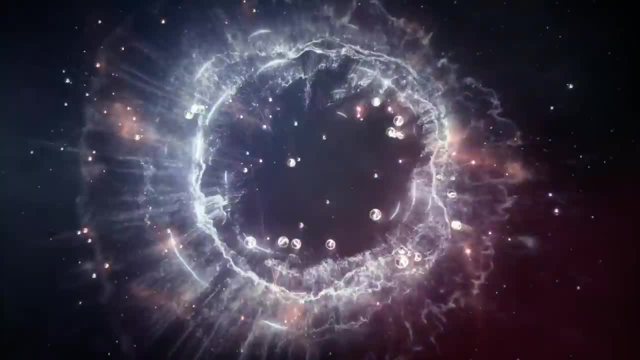 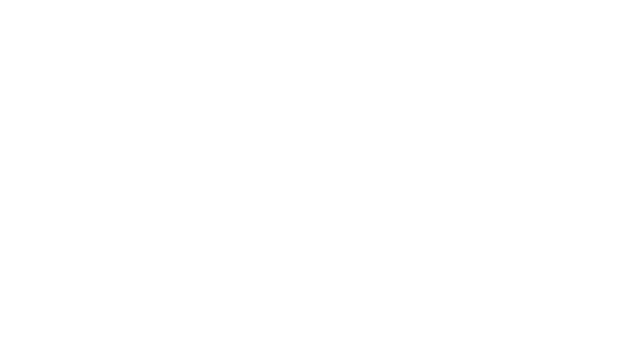 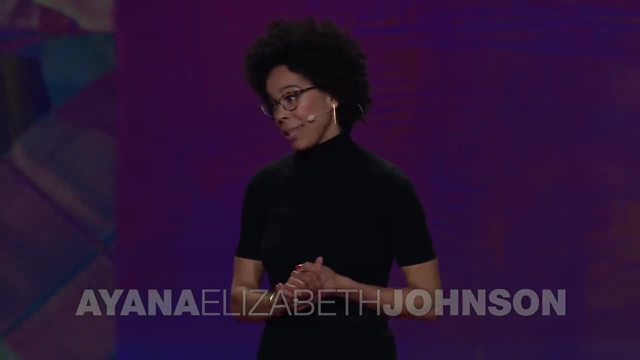 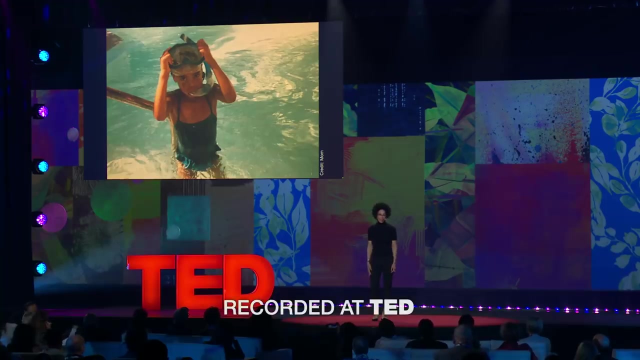 I want to tell you a love story, but it doesn't have a happy ending. Once upon a time, I was a stubborn five-year-old who decided to become a marine biologist. Thirty-four years, 400 scuba dives and one PhD later. 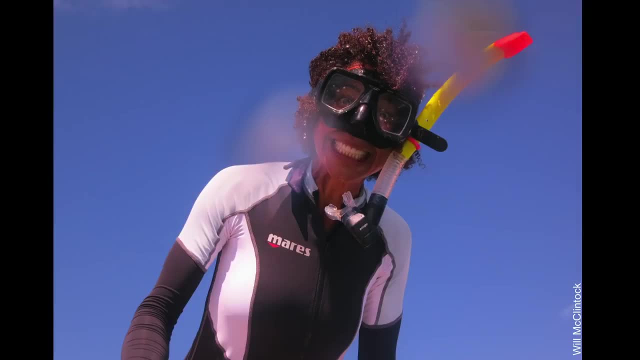 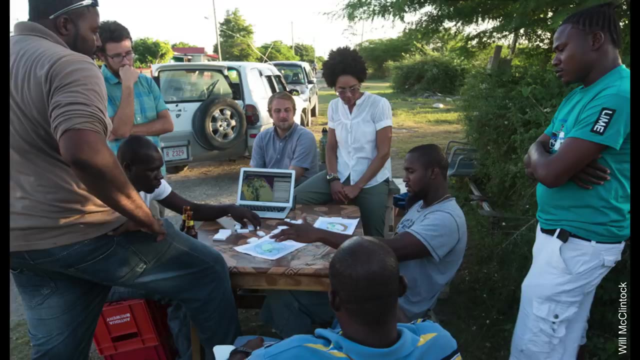 I'm still completely enamored with the ocean. I spent a decade working with fishing communities in the Caribbean counting fish, interviewing fishermen, redesigning fishing gear and developing policy. I've been helping to figure out what sustainable management can look like for places where food security, jobs and cultures 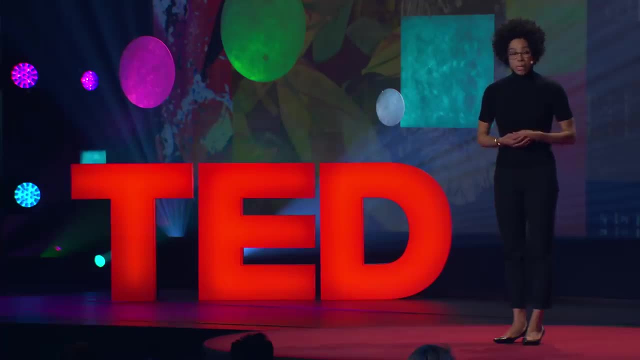 all depend on the sea. In the midst of all this, I fell in love with a fish. There are over 500 fish species that live on Caribbean reefs, but the ones I just can't get out of my head are parrotfish. 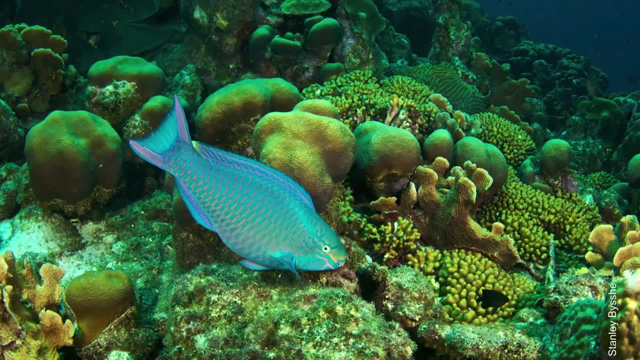 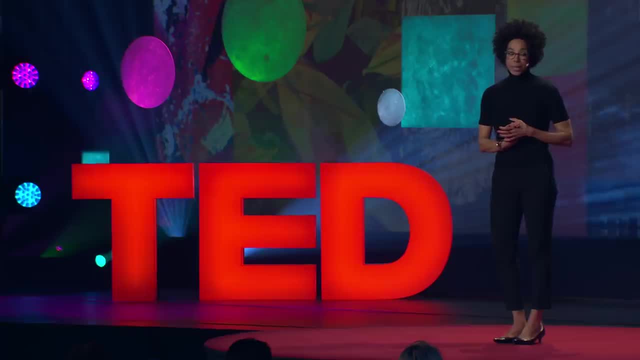 Parrotfish live on coral reefs all over the world. There are 100 species. They can grow well over a meter long and weigh over 20 kilograms. but that's the boring stuff. I want to tell you five incredible things about these fish. 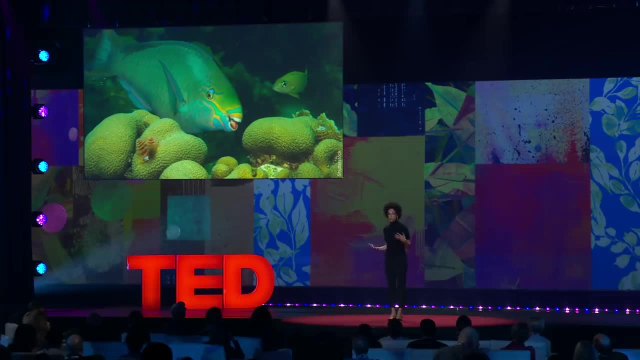 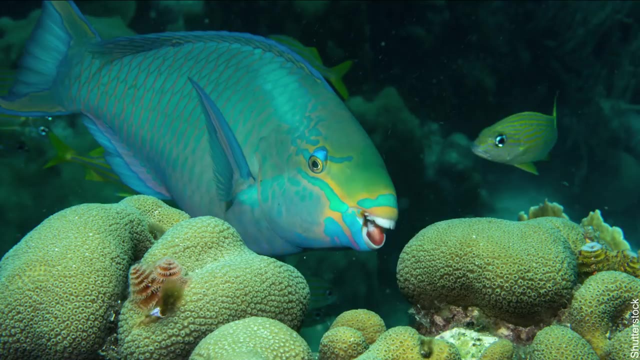 First, they have a mouth like a parrot's beak, which is strong enough to bite coral, although mostly they're after algae, They are the lawnmowers of the reef. This is key, because many reefs are overgrown with algae. due to nutrient pollution from sewage and fertilizer that runs off of land. And there just aren't enough herbivores like parrotfish left out on the reefs to mow it all down. Okay, second amazing thing: After all that eating, they poop fast. 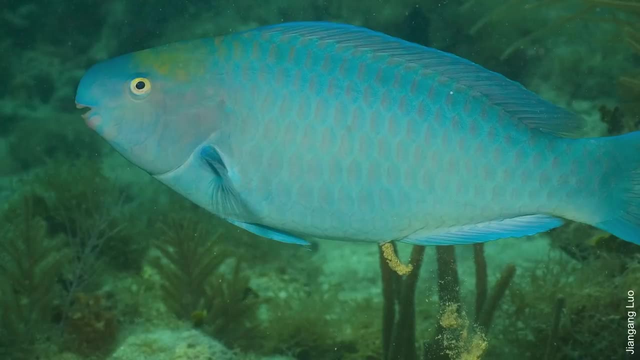 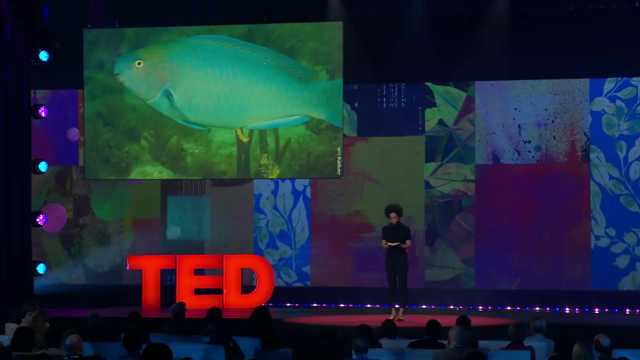 That's fine white sand. A single parrotfish can produce over 380 kilograms of this pulverized coral each year. Sometimes, when scuba diving, I would look up from my clipboard and just see contrails of parrotfish poop raining down. 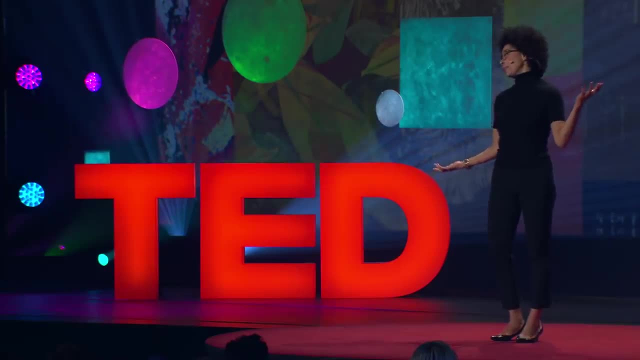 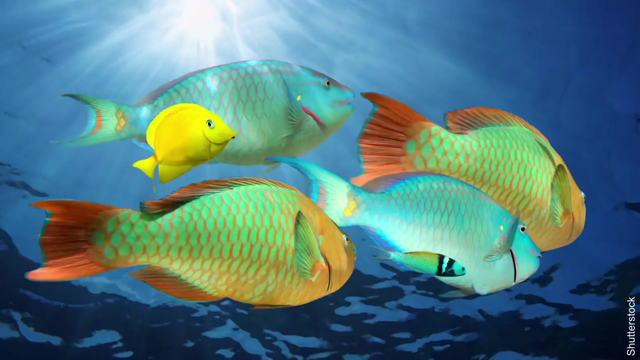 So next time you're lounging on a tropical white sand beach, maybe thank a parrotfish. Third, they have so much style: Mottled and striped. teal, magenta, yellow, orange, polka-dotted parrotfish are a big part of what makes coral reefs so colorful. 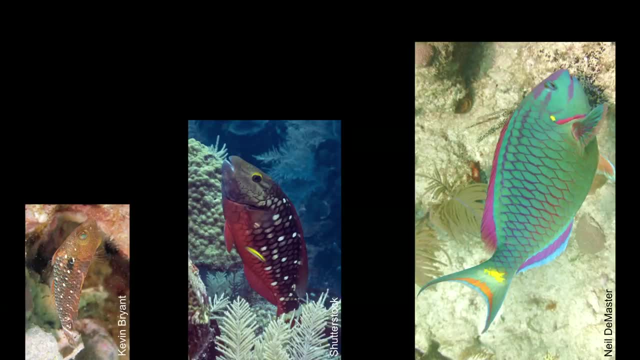 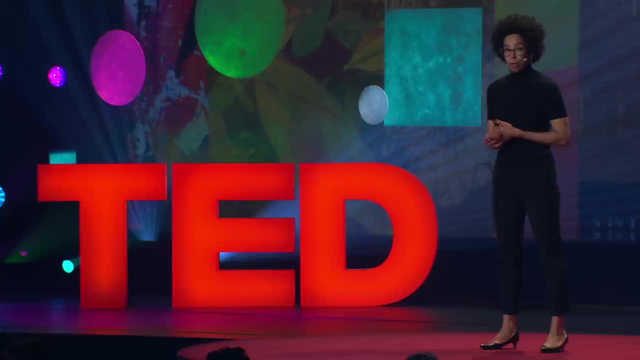 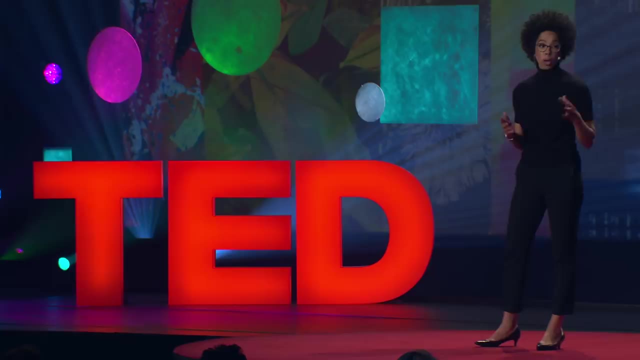 Plus, in true diva style, they have multiple wardrobe changes throughout their life: A juvenile outfit, an intermediate get-up and a terminal look. Fourth, with this last wardrobe change comes a sex change from female to male, termed sequential hermaphroditism. 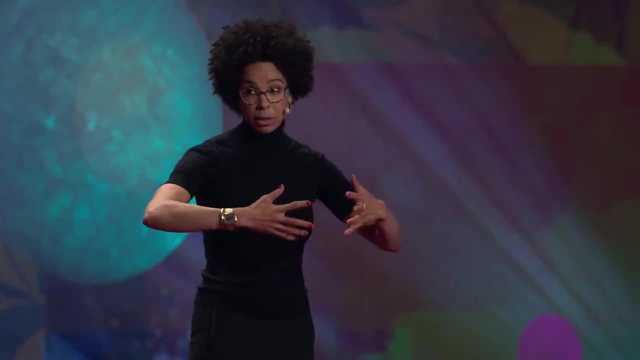 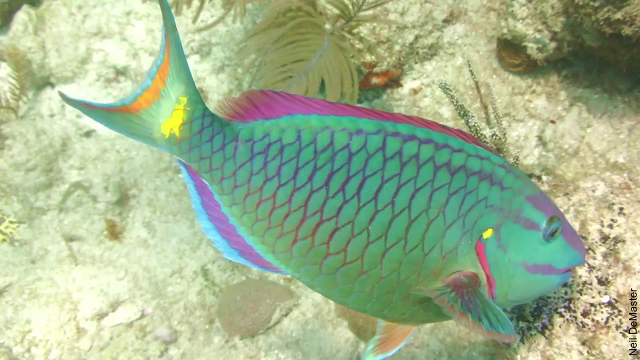 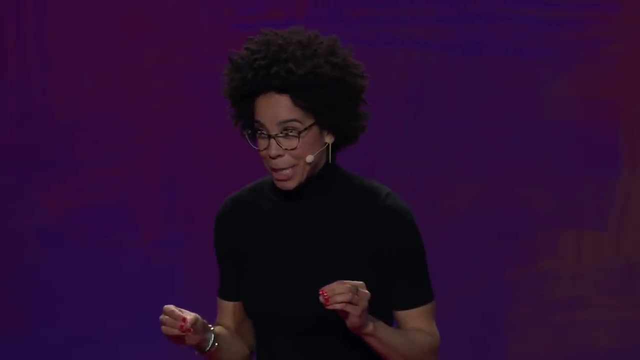 These large males then gather harems of females to spawn. Heterosexual monogamy is certainly not nature's status quo, and parrotfish exemplify some of the beauty of diverse reproductive strategies. Fifth, and the most incredible sometimes when parrotfish cozy up into a nook in the reef at night. 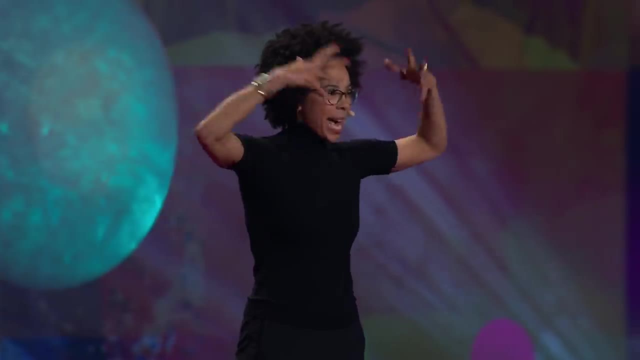 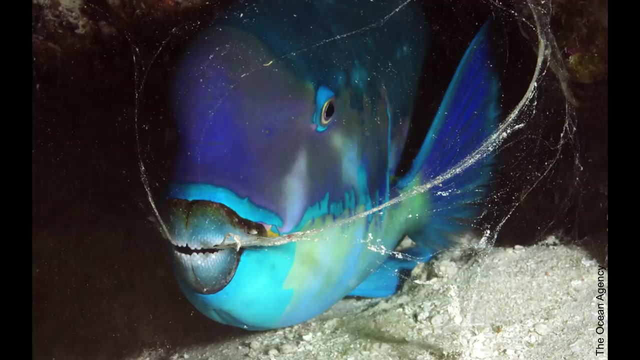 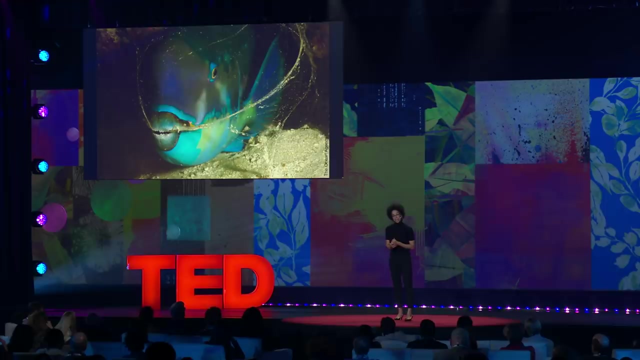 they secrete a mucus bubble from a gland in their head that envelops their entire body. This masks their scent from predators and protects them from parasites, so they can sleep soundly. I mean, how cool is this? So this is a confession of my love for parrotfish. in all their flamboyant, algae-eating, sand-pooping, sex-changing glory. But with this love comes heartache. Now that groupers and snappers are woefully overfished, fishermen are targeting parrotfish. Spearfishing took out the large species. 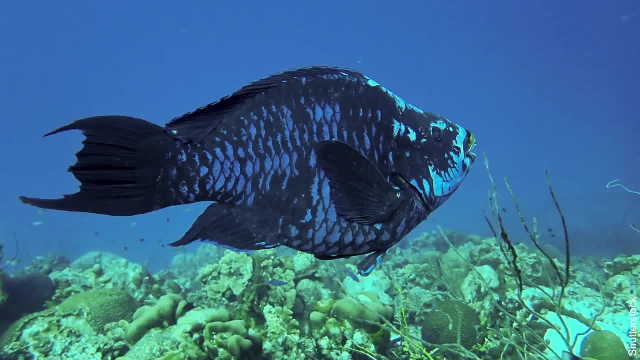 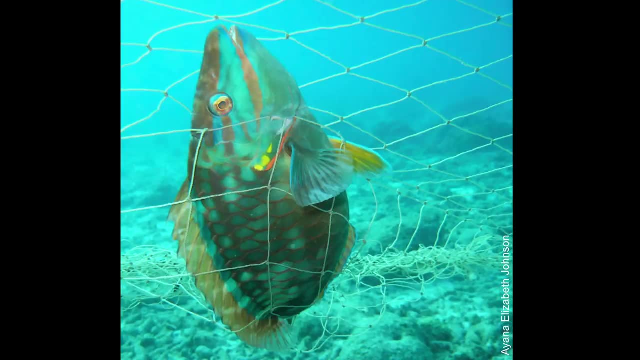 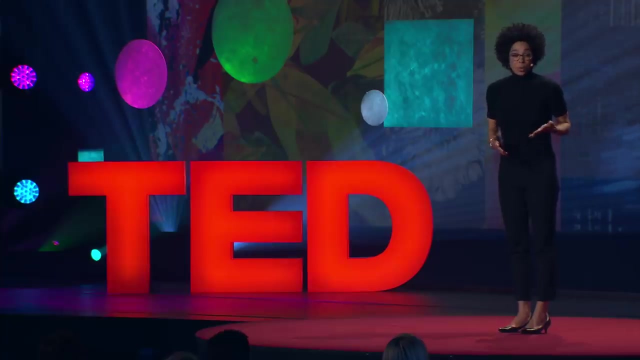 midnight. blue and rainbow parrotfish are now exceedingly rare, and nets and traps are scooping up the smaller species. As both a marine biologist and a single person, I can tell you there aren't that many fish in the sea, And then there's my love for their home. 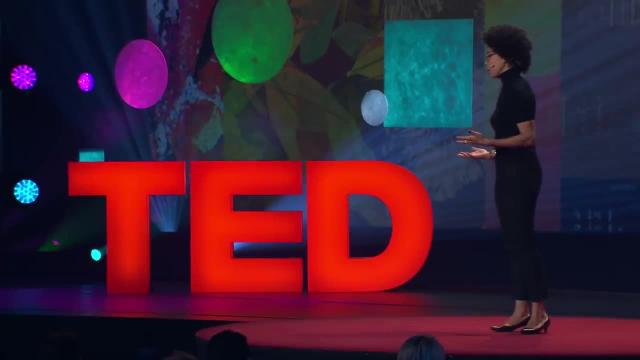 the coral reef, which was once as vibrant as Caribbean cultures, as colorful as the architecture and as bustling as Carnival. Because of climate change, on top of overfishing and pollution, coral reefs may be gone. within 30 years, an entire ecosystem erased. 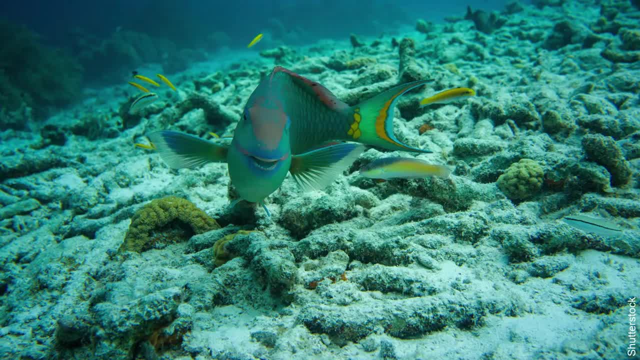 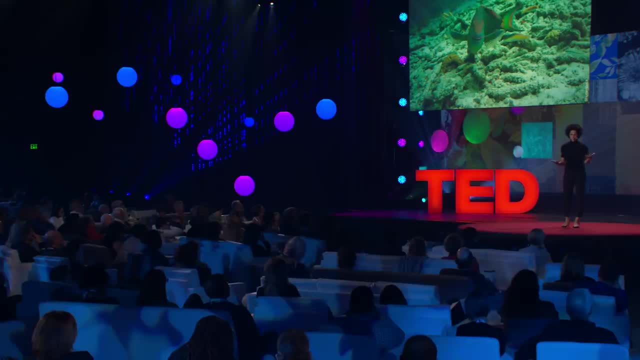 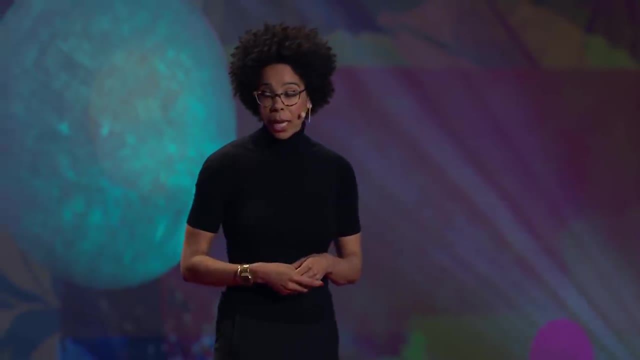 This is devastating because hundreds of millions of people around the world depend on reefs for their nutrition and income. Let that sink in. A little bit of good news is that places like Belize, Barbuda and Bonaire are protecting these VIPs- very important pairs. 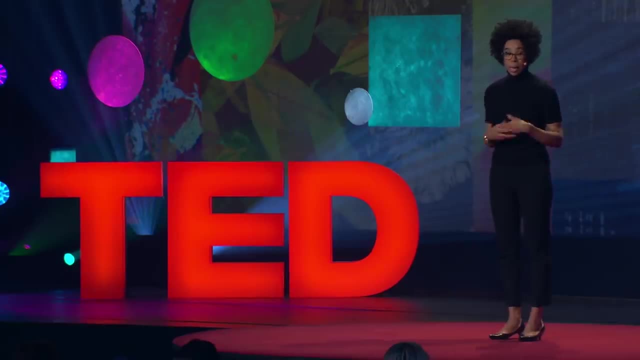 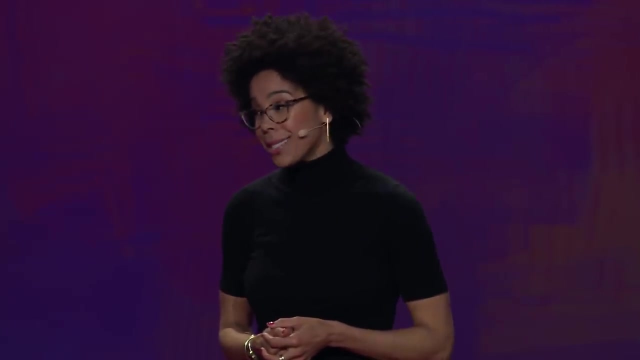 They're not just parrotfish. Also, more and more places are establishing protected areas that protect the entire ecosystem. These are critical efforts, but it's not enough. As I stand here today, only 2.2 percent of the ocean is protected.